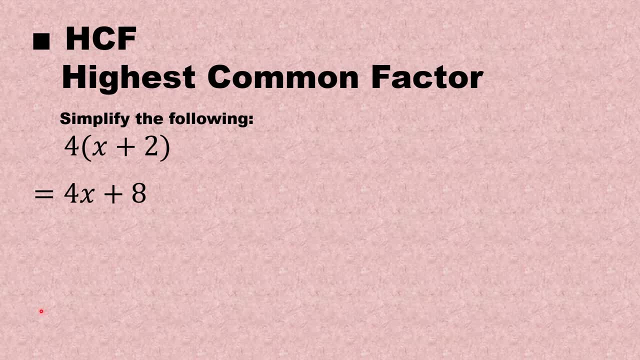 where you are going to start with four X plus eight and you're going to take out a highest common factor. So if I say to you, factorize the following and I give you the expression four X plus eight, then you're going to say what is the biggest number and what is the most variables. that 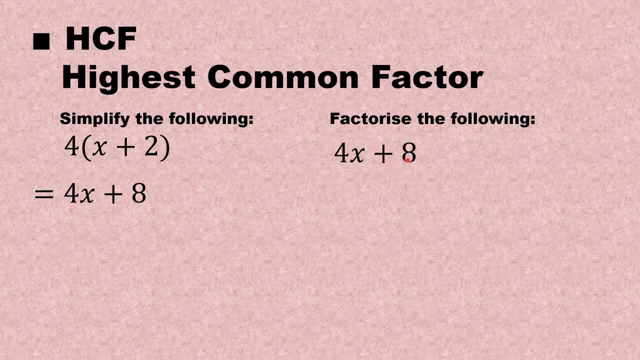 I can take out of both of these terms over here. So if you look at the four, the four and the eight, the highest common factor of four and eight is a four. So you can take out a four, and can I take out an X here? Yes, But can I take out an X there, No. 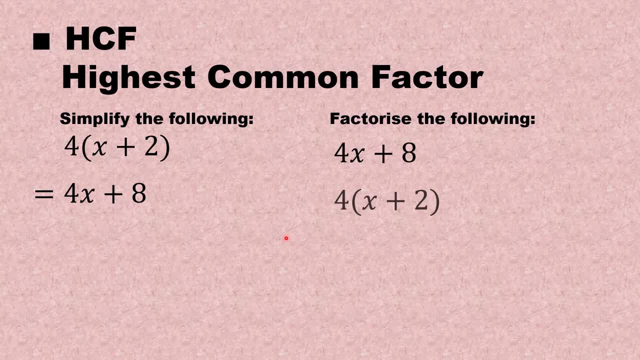 So you can only take out a number, and that would be four. So if you take out the number four, what you're going to do is you're going to divide each and every term because, remember, we distributed and we multiplied in. So what is the inverse of distributing or multiplying? 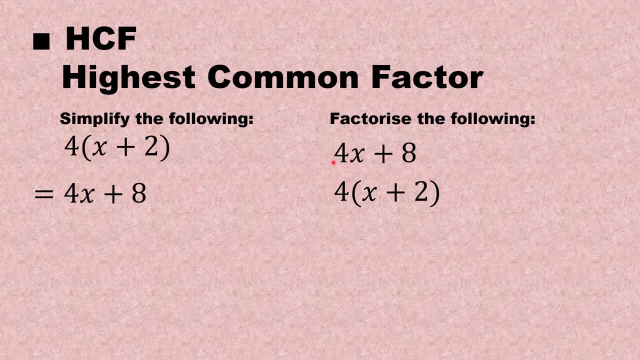 It's division. So, whatever you took out, you divide each term with that number. So you're going to divide four X with X. sorry, four X with four, And what is left, an X plus eight divided by four, is two. So that is the factorized form. So why do we do this? People always ask, but ma'am, 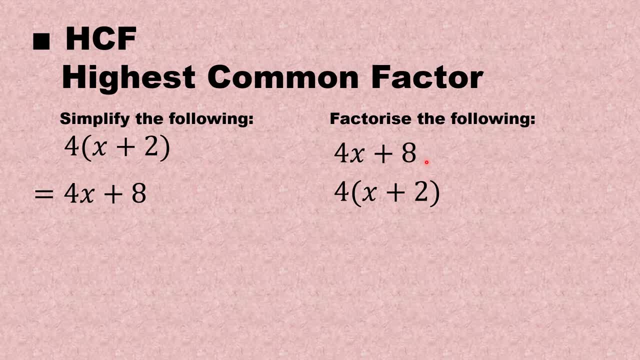 why do we go back and now, you know, do the inverse of this. now again, It's to simplify an expression more fully. Okay, Or so why do we do this? Let's just have a look. So if I say to you four plus two divided by two, please, people, if you can take out the number four, you're going to. 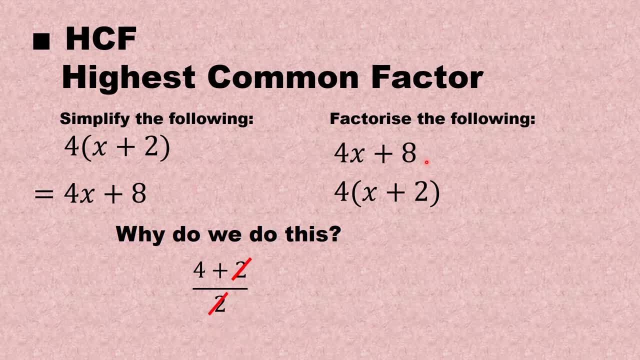 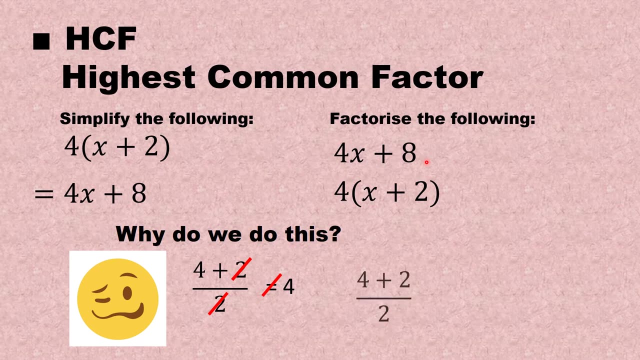 two terms on top of that fraction. You cannot just say, oh, the two divided by two, that cancels out. And my answer is four, because indeed four plus two is six. Six divided by two does not give you four, but it does give you three. Okay, So you cannot do that, But so let's. 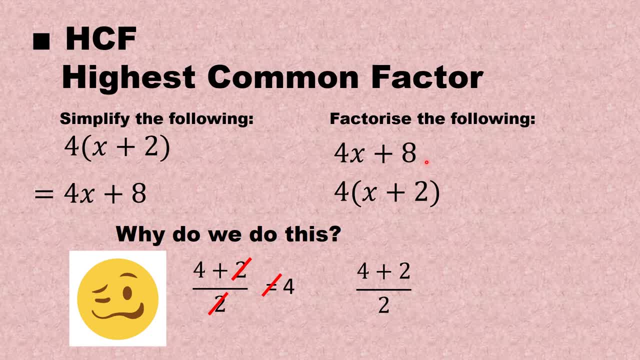 say if I take four plus two divided by two, and you can say: but ma'am, you can just simplify the top. But what if you add variables there and you cannot simplify the top? You want to simplify it because there's no way of adding the top. So you're going to factorize the top, So I'm going. 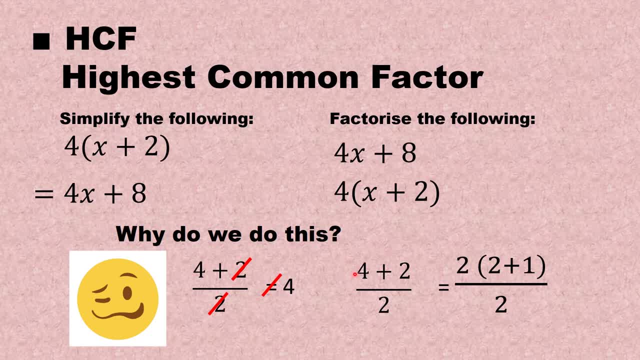 to take out a two. If I take out a two, with four plus two, I take out a two. Remember what you take out. you divide with every term and then that will give you what is left inside the bracket. So four divided by two gives you two, and two divided by two gives you a positive one. 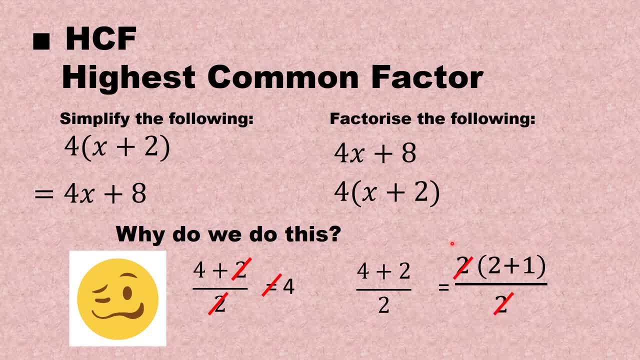 So now you can say: aha, I'm going to delete those two twos. Why? Because I created on top one term. Can you believe that this is one term? But then you say: oh, but ma'am terms are separated by plus and minuses. We've learned this in grade eight, or even in grade 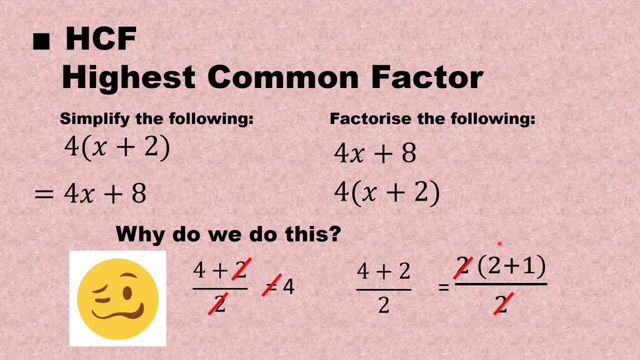 seven already, Okay. But then you say, remember, a term is separated by plus and minus unless it is inside a bracket. So now that becomes one term. So we've got one term divided by another term, and then you can cancel out. 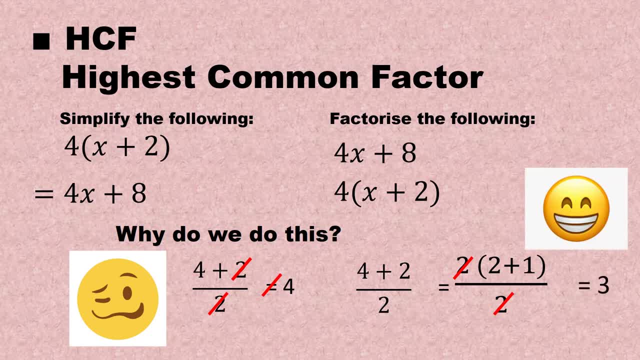 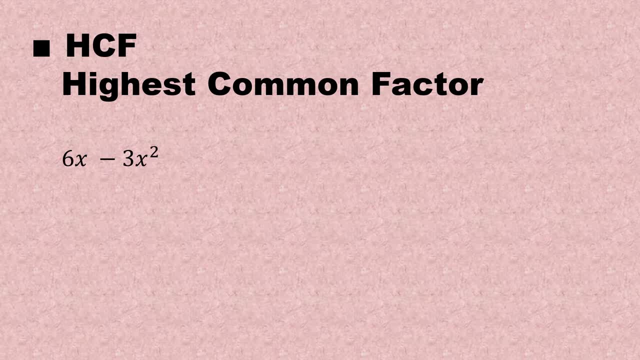 So you can cancel out there. And then your answer is three, which is correct. Okay, Let's have a look at a few examples with the highest common factor, All right, So please remember, if you cannot see one of the others, your first port of call is to see whether you. 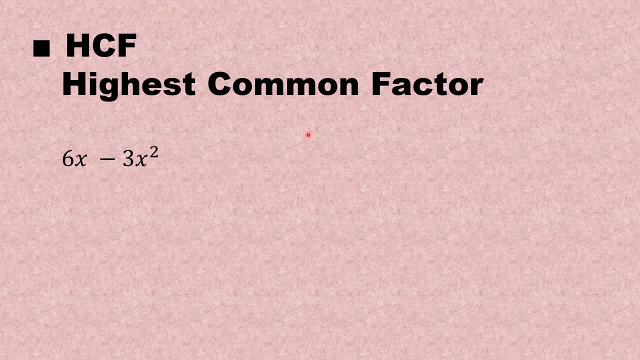 can take out a highest common factor. So it's very important that you understand this Right. Let's have a look at these two terms. What can I take out from both of them? Okay, So if you look at the numbers first, there's a two. So if you look at the numbers first, there's a two. So if you 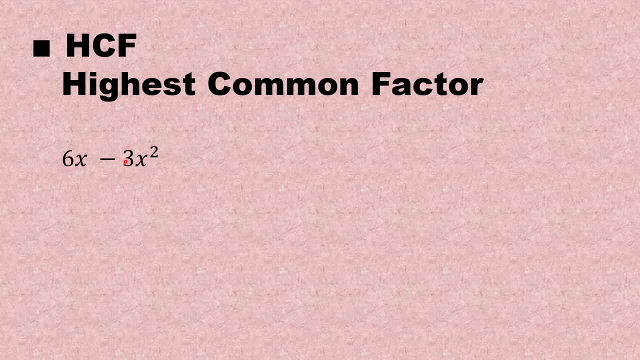 look at the numbers first. there's a three and there's a six. So the highest number you can take out there is a three. Then you go to this term. You say, oh, there's two X's there Can I take. 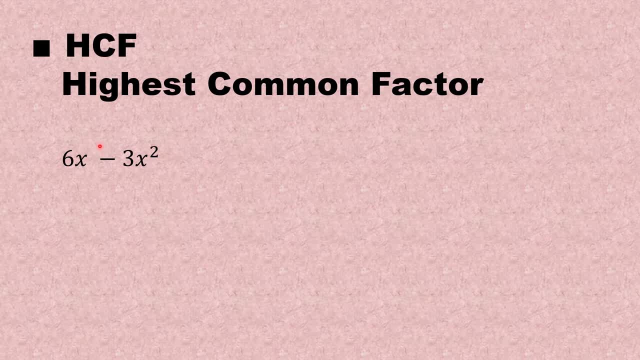 out two X's from both of them? No, because this one only has one X. So then you ask yourself: can you take out one X from both of them? Yes, So the highest variable you can take out there is one X. So you normally go with the one with you take the variables and the one with the lowest. 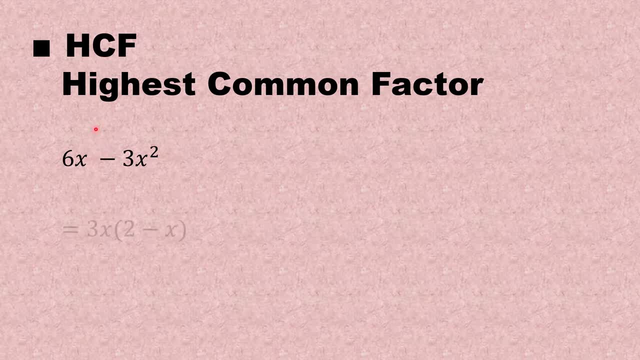 exponent: Okay, So we're going to take out three X, So three X. you divide it. So that's six X divided by three X, Six divided by three is two, and X divided by X is one. Two times one stays two Negative divided. 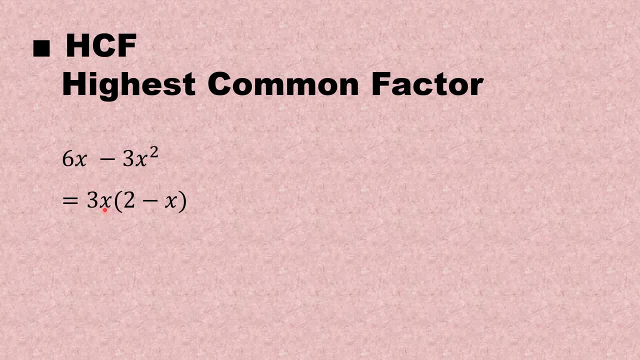 by positive is a negative. X squared divided by X is a X. So there, you fully factorized that expression. Okay, Let's have a look at this one. No variables there, So you can't take any variables out. but I can go and take out a nine. So you can take out a nine. So you can take out a nine. So 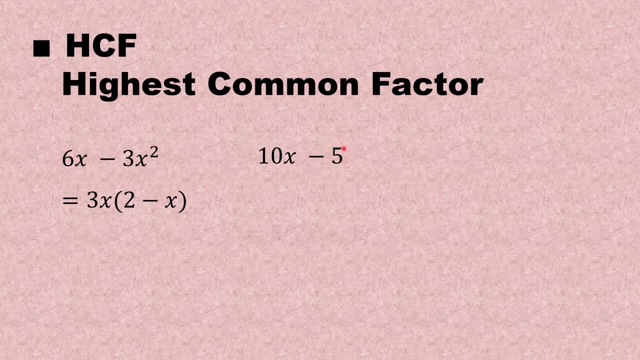 they're both multiples of five, So I can take out a five. and what is left? 10 X divided by five is two X Negative. five divided by five is negative one. There you fully factorized. Okay, Variables not the same, So you can't even think of taking one out, but I can. there's a six and a nine. 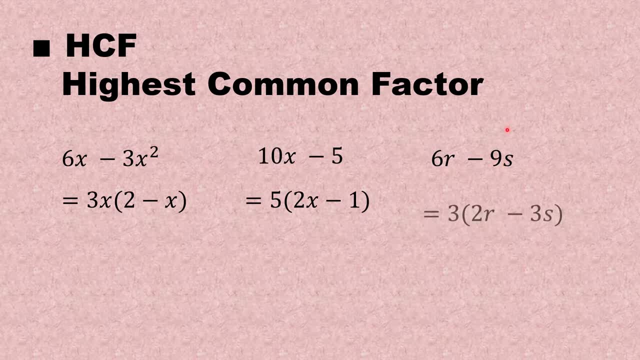 What are factors of six and nine? It is three, Okay. So you take out a three. six R divided by three is two R. Negative. divided by positive is a negative. So you can take out a nine, So you can negative. nine divided by three is three S Okay, Fully factorized. Let's have a look at this one. 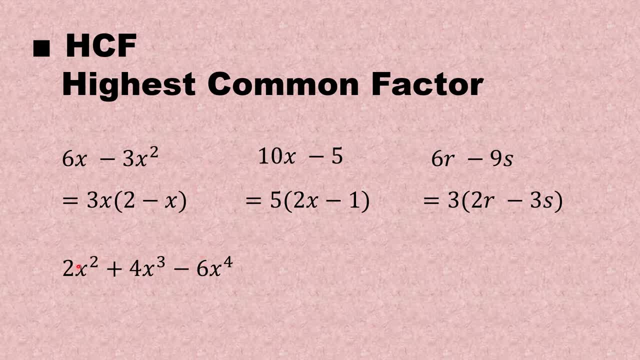 Easy to see the numbers. The biggest number you can take out there from all of them successfully without leaving a fraction or an integer number- Sorry, not an integer, a fraction. You must be left with a whole number. Okay Is two, So you can take out two over there. 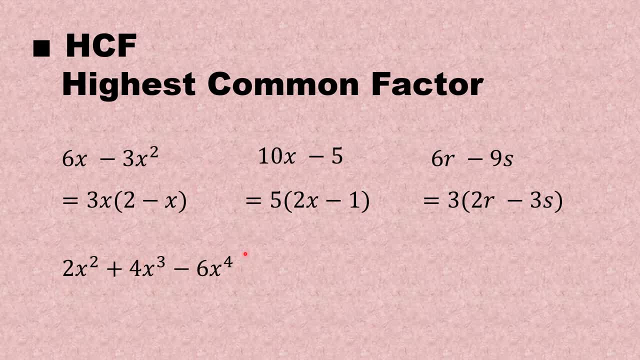 I can take out two from everyone. So how many X's? This one's got four X's. This one's got three X's. This one's got two X's. So what is the most X's that you can take out from all of them successfully? 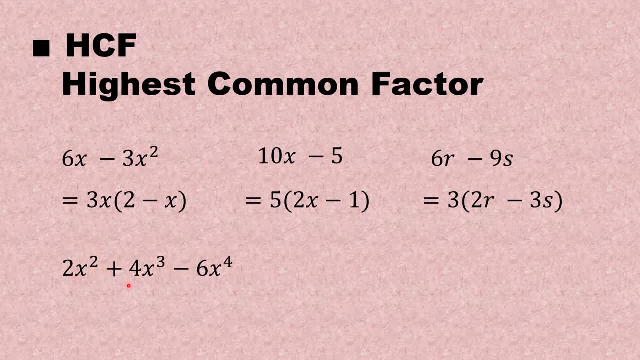 is two X's. Okay, Can you see all of them have two at least. All right, So I'm going to take out two X squared. So you take each and every term and divide with what you've taken out. So two X. 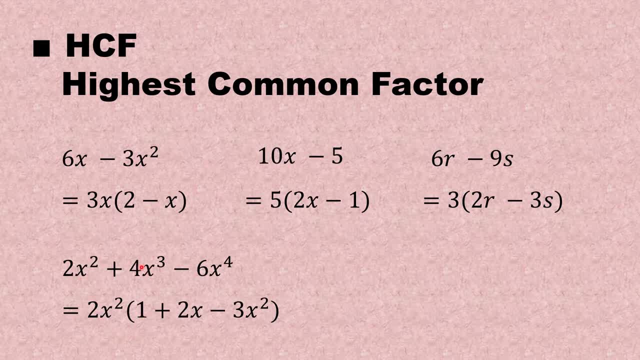 squared. divided by two, X squared is one: Four, X to the power three. divided by two: X squared, Four. divided by two is two: X to the power three. divided by two, X squared is one: Four, X to the power three, X to the power two. Remember, if you divide you minus those exponents. So three minus two is one. 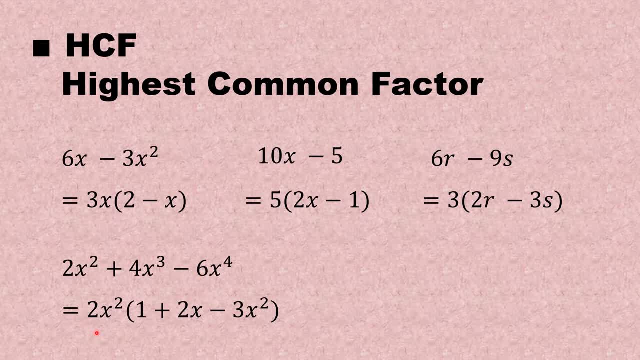 Negative divided by positive is a negative. Six divided by two is three. X to the power. four divided by X to the power two gives you X to the power two, And there it is fully factorized. Last one: Okay, Take out a five. How many X's? Four of them, Okay, Can you see immediately that? 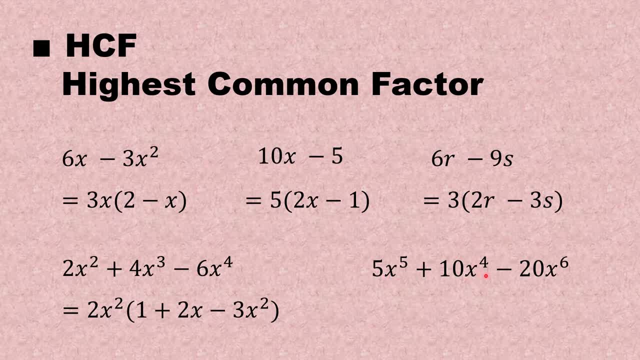 one's got six, This one's got five, This one's got four. So the most that I can take out is four. So I'm going to take out five X to the power four. Divide each term with that term that you've taken out. Five X to the power four divided by five X. sorry, five X to the power. 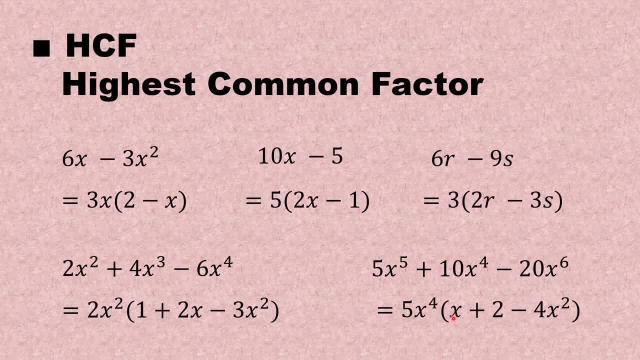 five divided by five, X to the power four is just an X plus 10 divided by five is two. X to the power four divided by X to the power four is one. Two times one just stays two. Negative divided by positive is a negative. Twenty divided by five is four. And then you take out five X to the power. 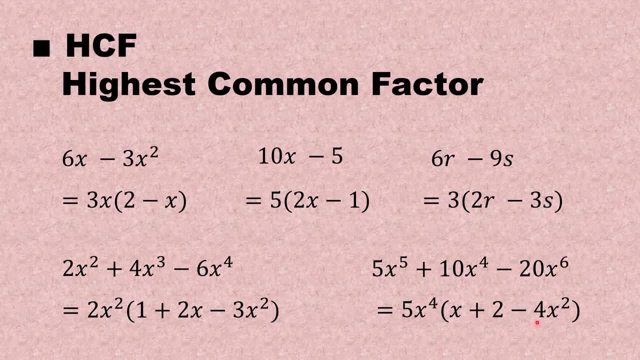 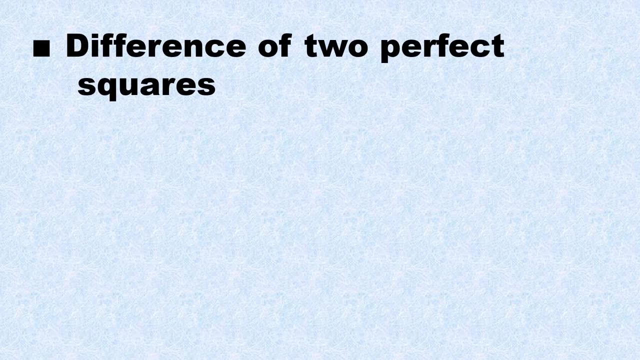 six divided by X to the power four is X to the power two. Okay, And there it's fully factorized. I hope you understand the highest common factor And if you don't, otherwise, after this please reach out to your teacher. Okay, Okay, Let's move on to the difference of two. perfect. 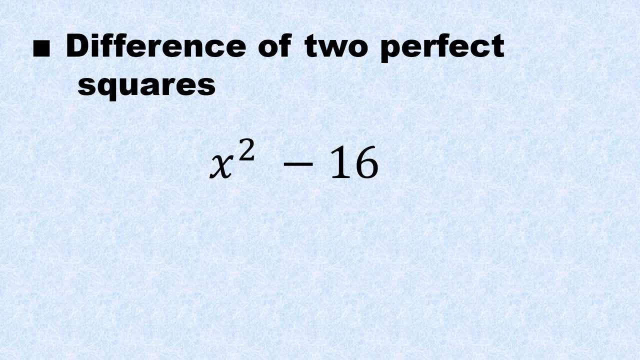 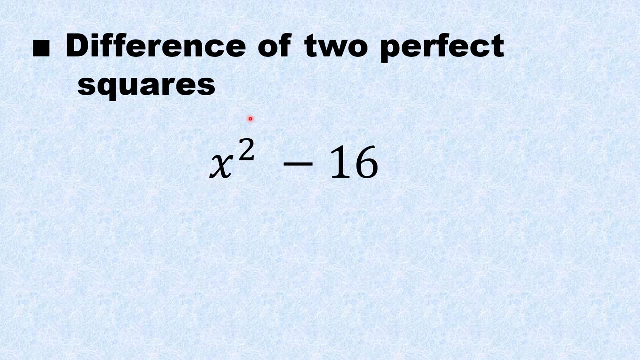 squares. So the hint is in the name. It's the difference, which means it's a minus of two perfect square rootable numbers on each side. So very important Has to you have a minus in the middle and both sides has to be perfectly square rootable And that is why. 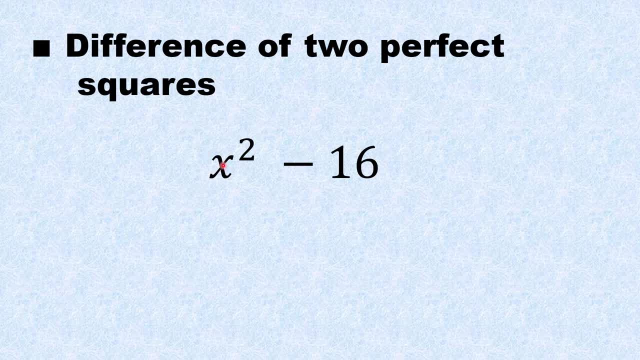 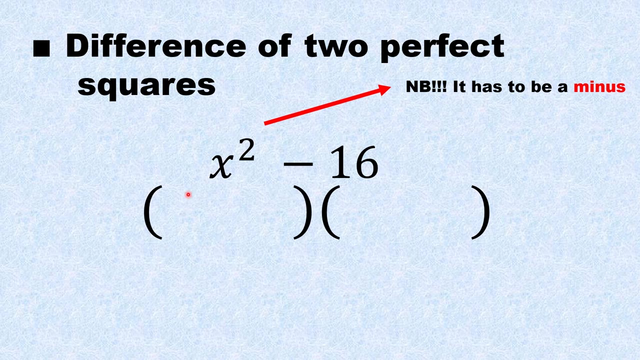 we taught you how to square root with an exponent And remember how do you do that inside over outside, so that you can factorize now. Okay, So very important. NB, it has to be a minus. You always set up your two brackets always, and it's always in the middle there And it doesn't. 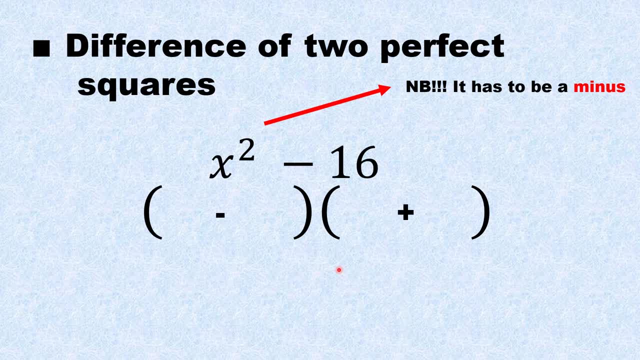 matter which one comes first, A minus or a plus, or a plus and a minus. Okay, For the first part. in your two brackets, that first space, you square root X to the power two, The square root of X to the power two gives. 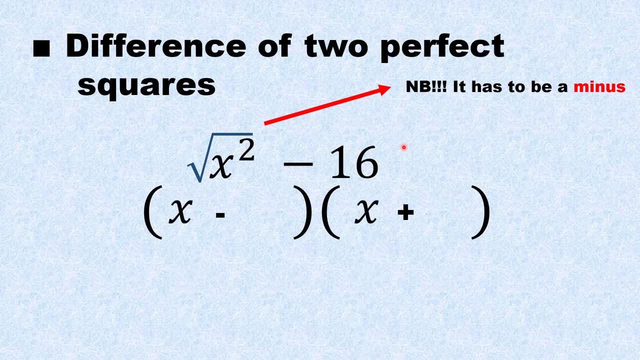 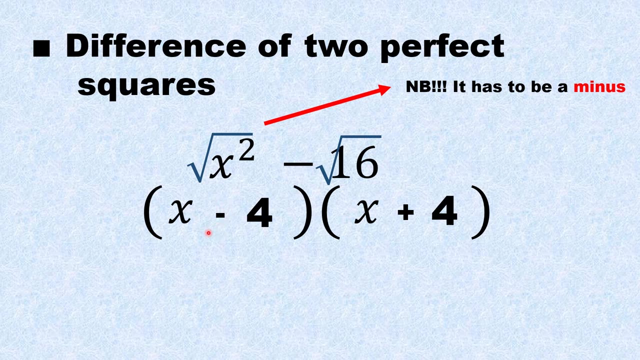 you X and X. The square root now for the second term takes the second space. The square root of 16 is four and four. Okay, Right, So exactly the same. Your brackets are going to look exactly the same. Instead, in the one, there's going to be a minus and the other one, there's going to be a plus. 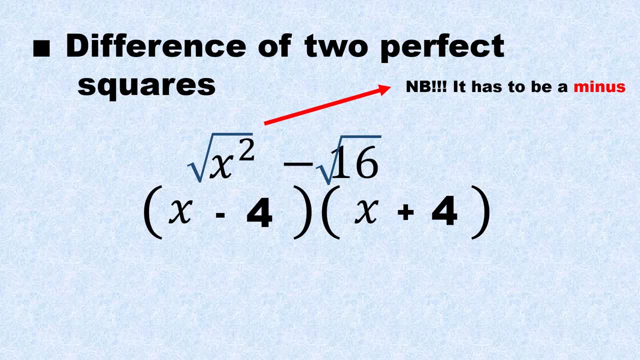 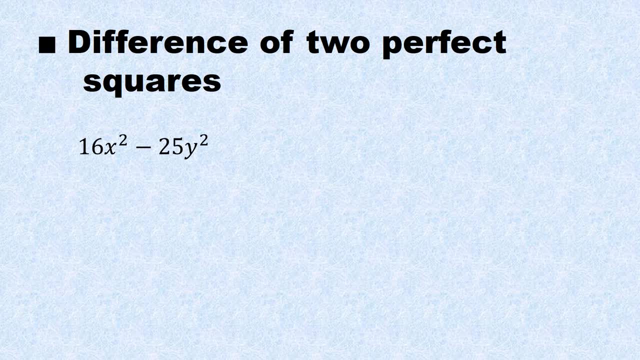 And again, it doesn't matter which one comes first. All right, Let's quickly have a look at a few examples. Okay, Immediately, if you see two terms, two terms with a minus inside, you think: isn't this a difference of two perfect squares? And if they're not perfectly square, rootable? 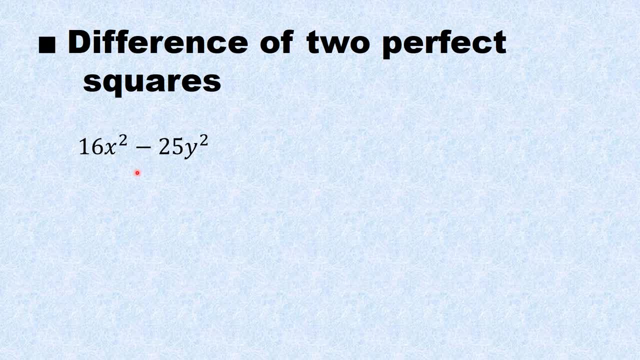 ask yourself: can't I take out an HCF first and then do a difference of two perfect squares? Okay, But let's just have a look. These are all straightforward Difference of two perfect squares examples. So can I perfectly square root 16, X to the power two, 16.. Remember. 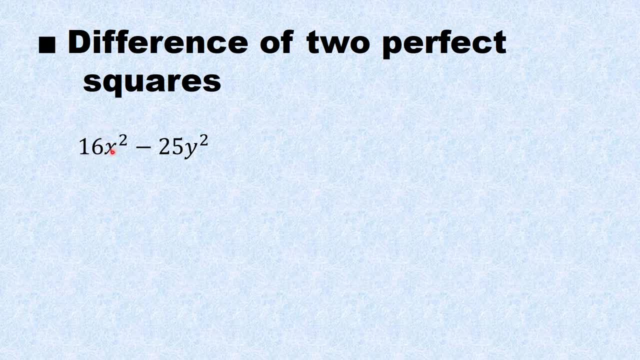 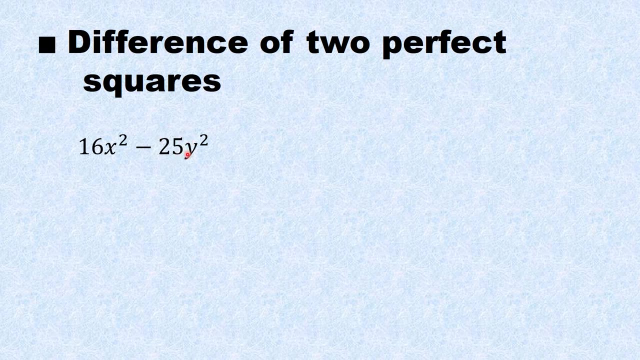 the number you square root as normal, and the exponent is inside over outside, So it's going to be four: X. Yes, And can I square root 25? Y squared? Yes, The number as normal, 25 squared, is five, and Y, squared inside over outside, is Y, So always two brackets. 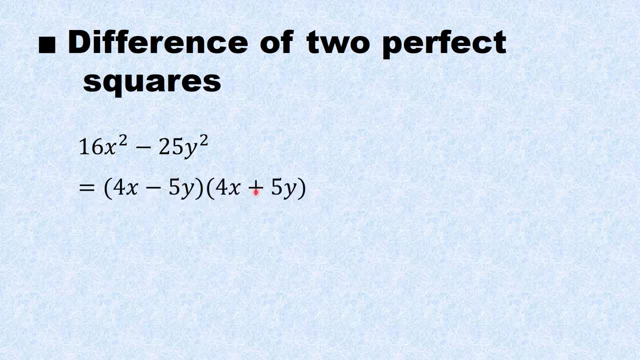 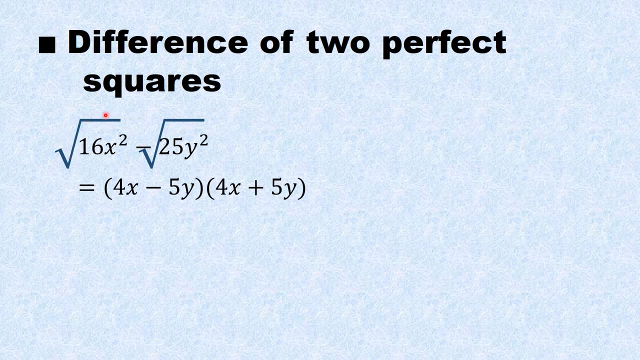 Minus, plus or plus, minus, it doesn't matter. And you square root that number. that takes the first position. square root that number takes the second position. Okay, Just to show you again, remember, it's the square root. So the square root of 16, X squared, is four. X takes up the first. 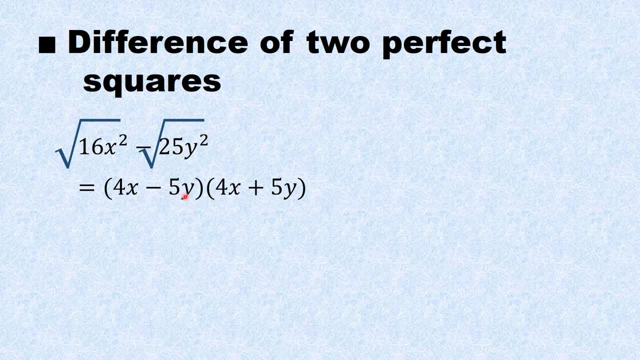 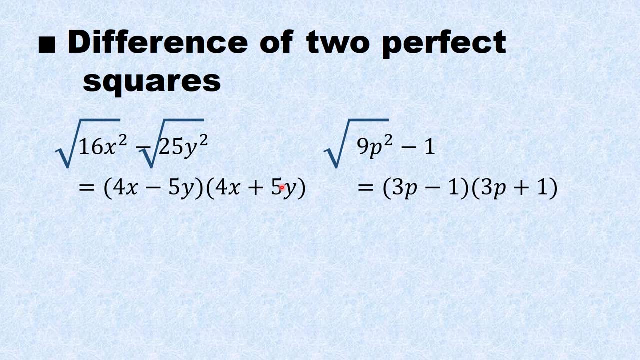 position and the square root of 25, Y squared, is five. Y takes up the second position. Okay, Let's have a look at this example. So please remember a one. If you see a one, a one, the square root of one is one. So if you see a one, 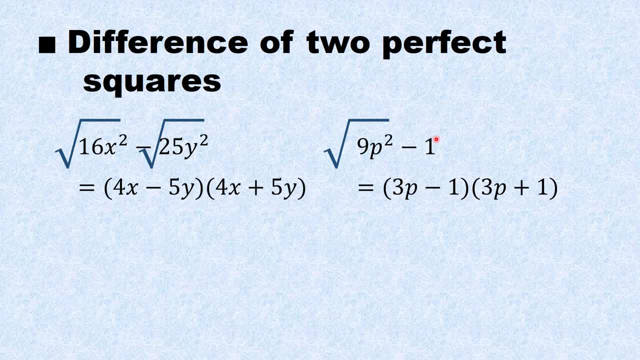 it's most definitely a difference of two perfect squares. Always remember, keep that in the back of your mind- that the one is a perfectly square rootable number. Okay, So two brackets minus plus. in your first position you're going to square root the first term there. nine P to the power. 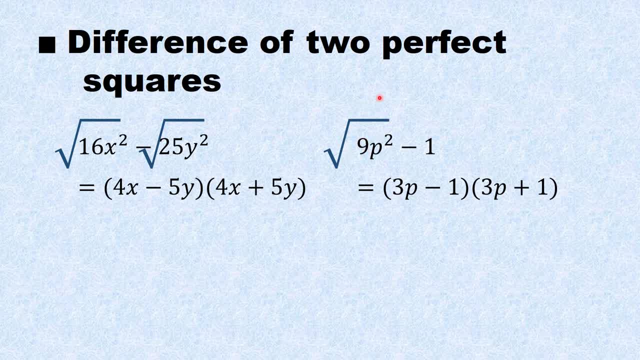 two, the number as normal. What is the square root of nine? It's three and P to the power two inside over outside. So if you see a one, you're going to square root the first term there: nine: P to the power two inside over outside. Two divided by two is one, So it's just P and then